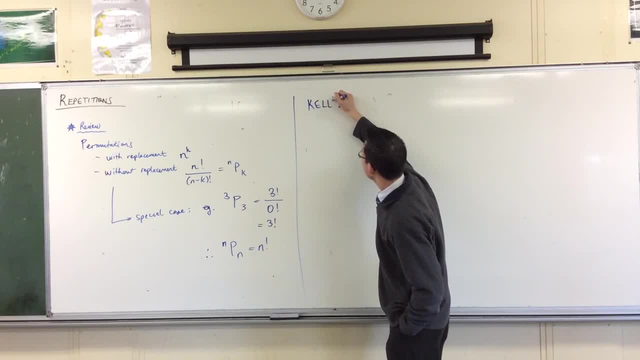 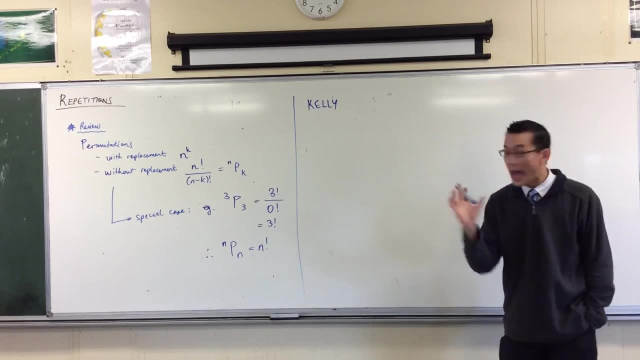 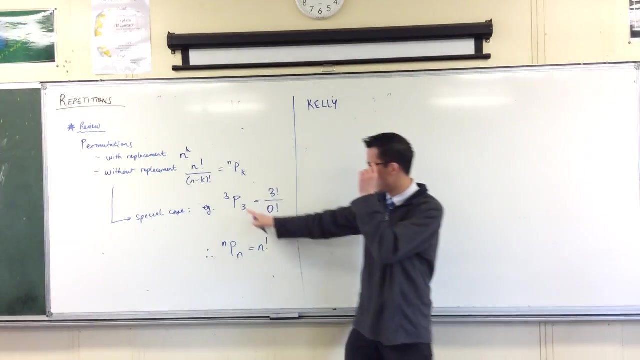 Kelly is a perfect name to pick. There we go. I picked this very specifically. Maybe you can work out why, as we go through Now, if I have here five objects and I want to arrange them and I want to arrange all five, so I'm in this kind of scenario. 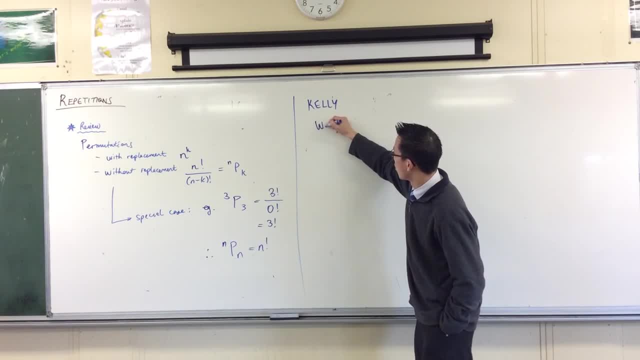 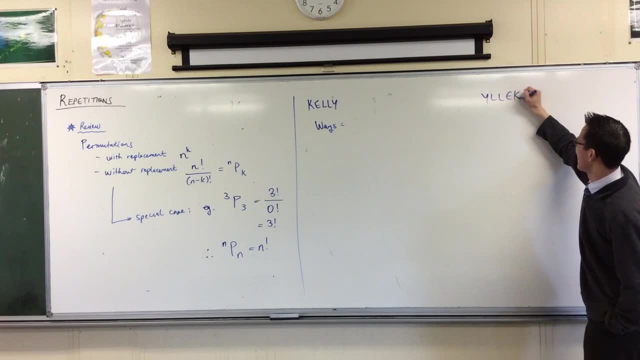 The normal thing you would say is: look, I've got the number of ways or the number of. they call them words, even though you know you're like it's not a word but it's a stringing together of letters. 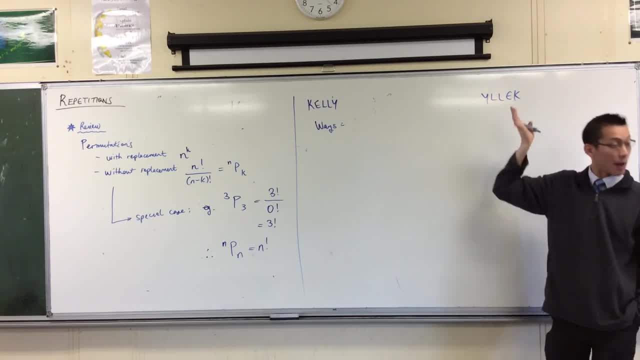 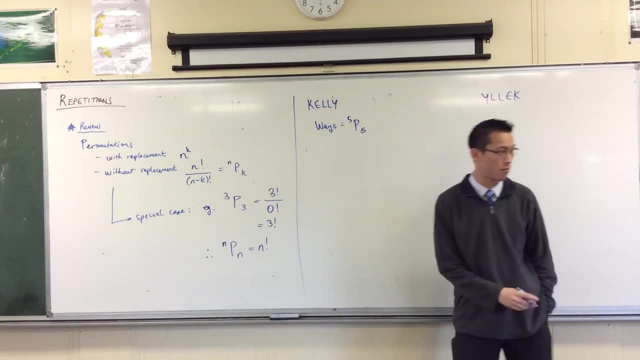 It's a word. Okay, How many ways can I arrange it? How many words do I get? And the first response you would say is: look, you're going to get five to choose from and you want to pick five of them, right? 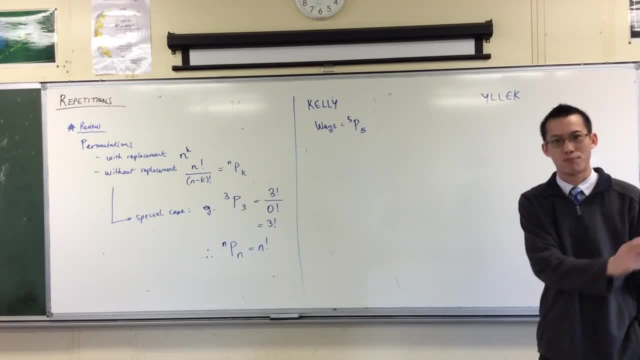 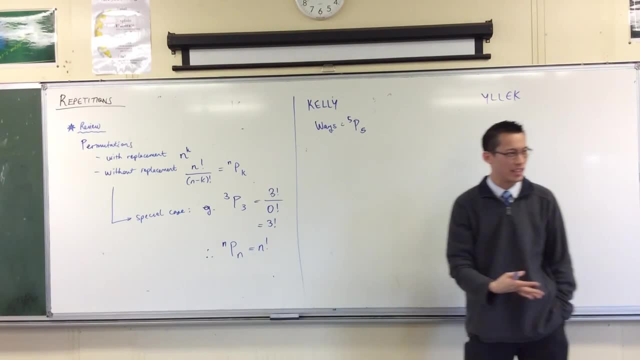 Five between five. so that's five factorial, okay, But there's a problem, right, Because of these repeated letters, because of these repeated letters, right, Actually, some of these arrangements, if I listed them all out, right, I'll get five factorial. 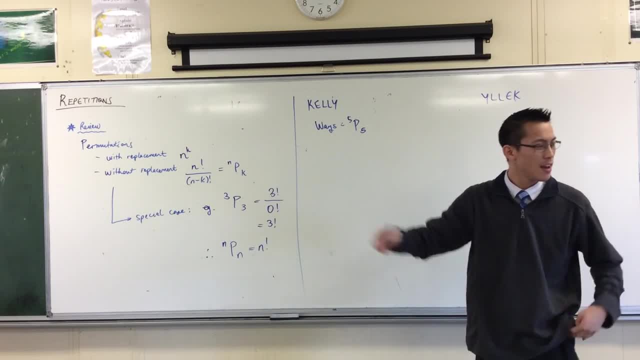 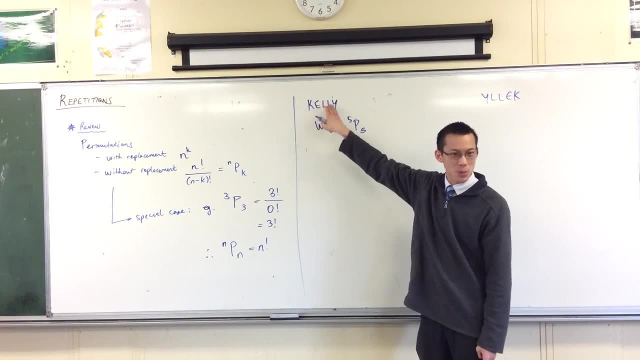 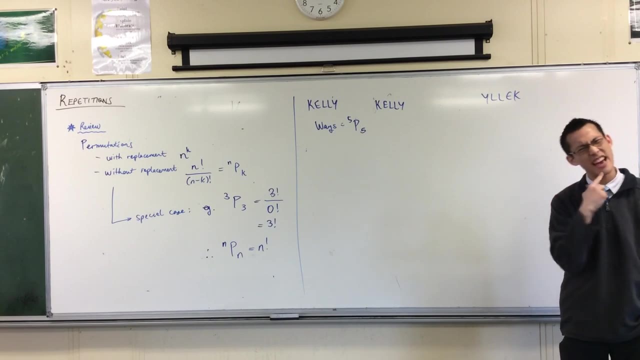 What's that? A hundred and twenty? A hundred and twenty, I think, right. But of those a hundred and twenty, some will look exactly the same. For instance, here's one arrangement right Now, if I switch the L's around, that's another arrangement, right. 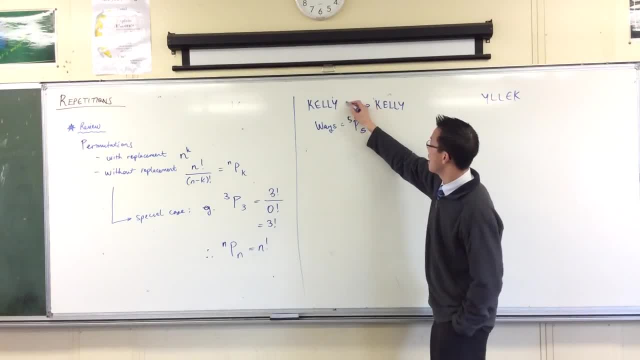 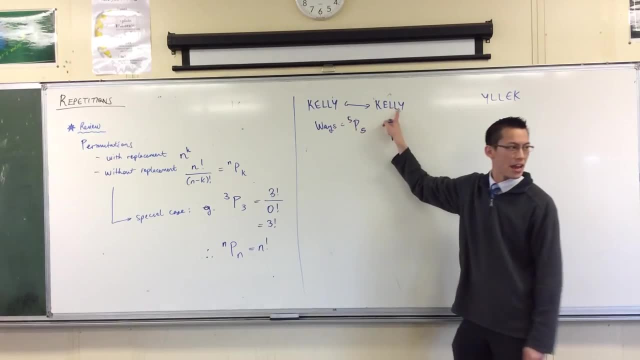 But it's not really, is it? It's not distinct, right? They're actually the same arrangement. So I've overcounted, right, I've overcounted. Now here's the thing: This is not the only double up that I've got, right. 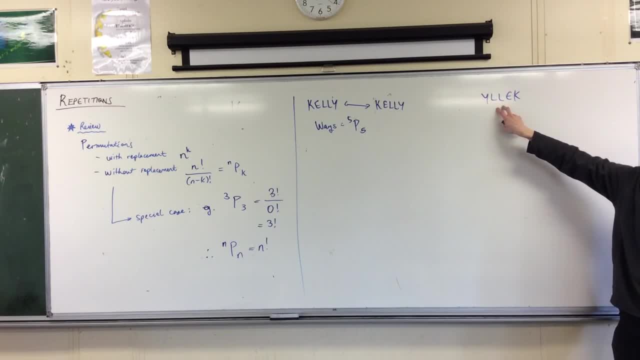 For example, let's go over here, right? I can switch the L's again, right, But I end up with the same word, right? So I've doubled up. In fact, every single one will have its double right. 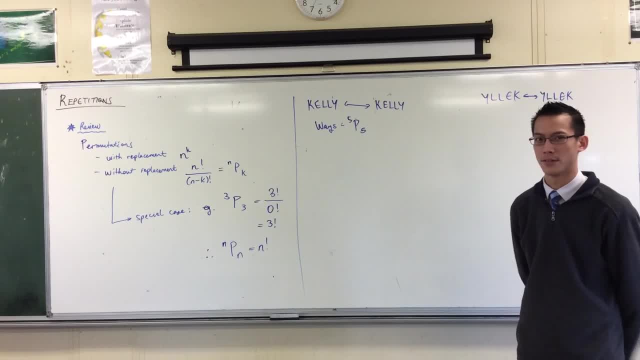 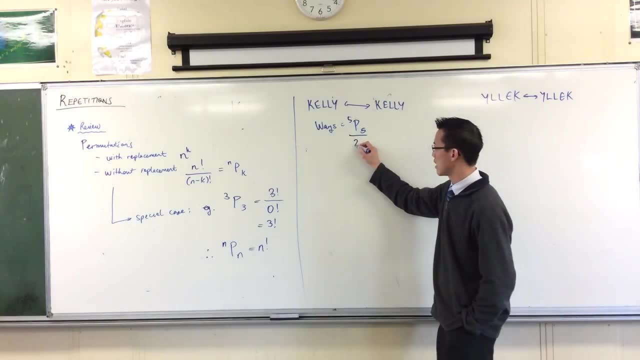 I've got twice as many arrangements as I really should have, okay, So to account for that, I need to divide by Now. I want to divide by two. That'll give me the right answer. okay, But there's actually more going on here. 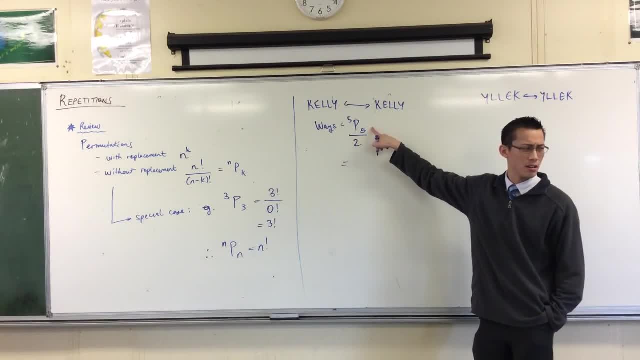 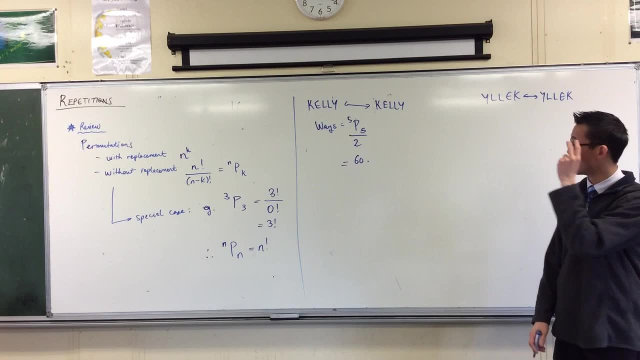 And to show you why, let's just write down what the number is. I think I said that was 120.. You can check it on your calculator. That gives me 60 different words. okay, There's more going on here, okay. 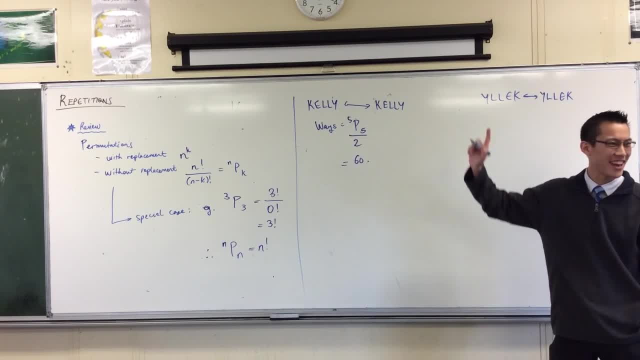 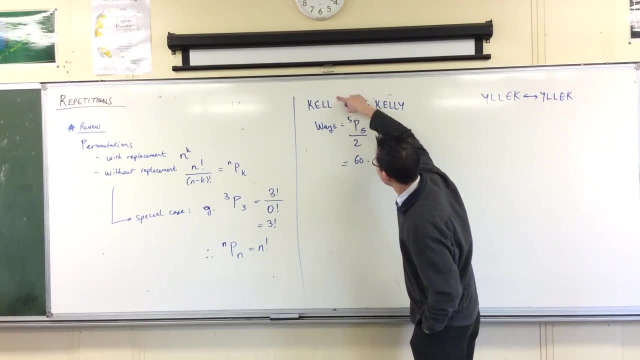 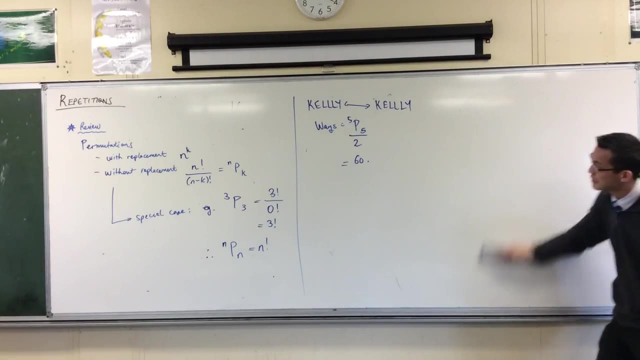 Let's give an example. Let's change Kelly's name. Sorry, Kelly. okay, I'm going to make there be three L's. So Kelly And I'll rub off these guys Right Now. think about this with me now, okay. 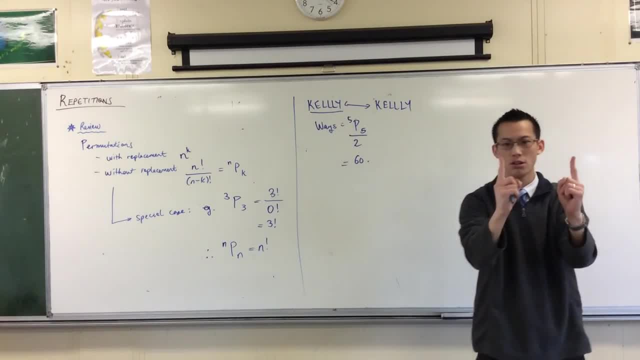 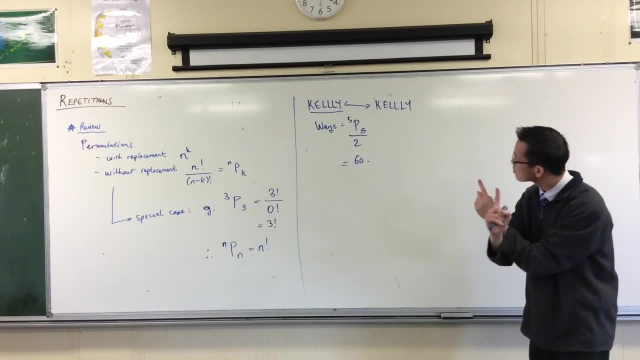 Here's one arrangement right Now, before when there was just two. okay, There's only one other way to rearrange the L's, And that is to swap, right. But just picture, Just picture the L's is, you know, as siblings, as triplets, right? 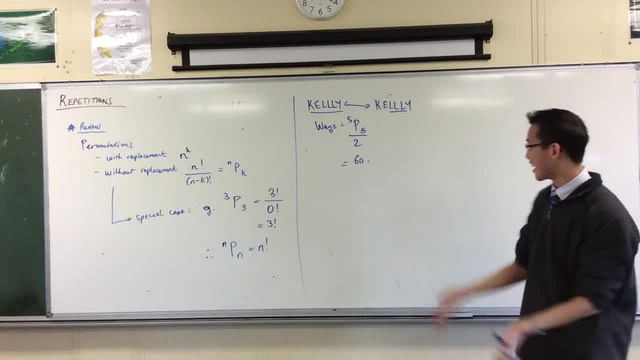 So the rest of us, if they're identical, triplets, right. We can't tell the difference, but they can, of course, right? So you know, I don't know if you have any friends who are twins, who, like you know. 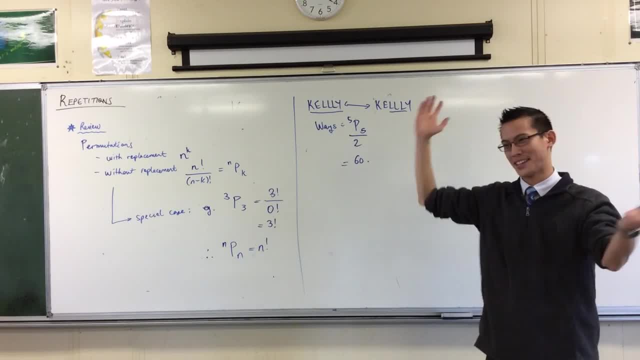 One day I just decided to Tie my hair up like this And we just swapped places all day Because I was bored of my classes. Sorry about that, But these guys right. The point is they can rearrange themselves without us being able to tell the difference. 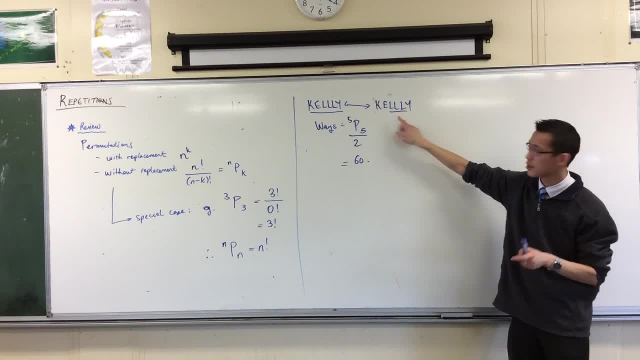 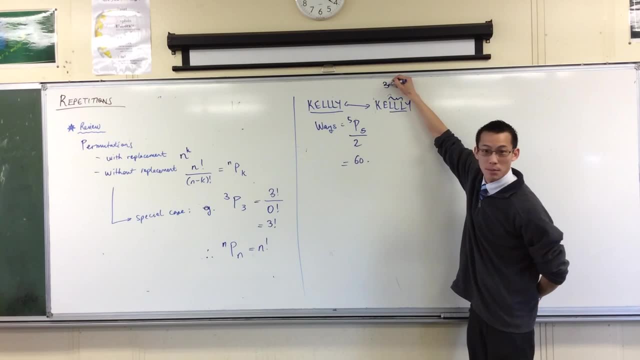 Does that make sense? Okay, Now think of the triplets. How many ways can I rearrange the triplets? And the answer is: I have three things to pick from And I want to permute them in three different ways. So that's going to be three factorial right. 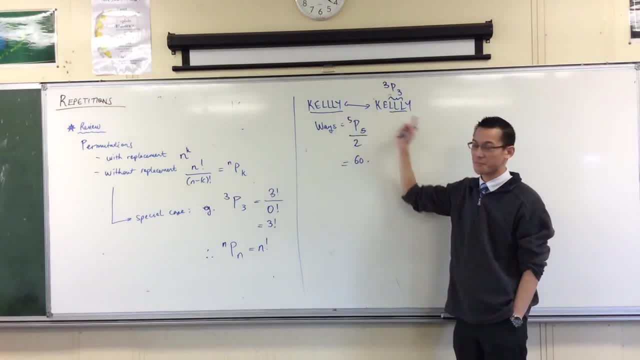 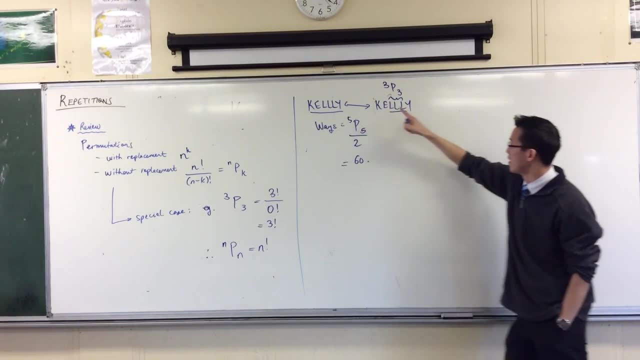 So, in fact, it's not just that I have, It's not just that I have three extra ways, right, I have three factorial extra ways. Every time I've got, you know, I've got this one, and then this one, and then. 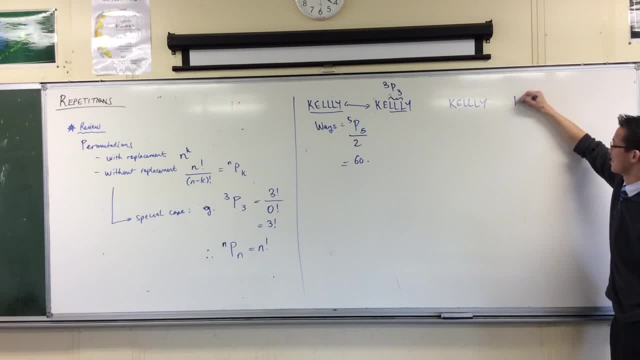 And then this one where they've rearranged themselves, which I still can't tell the difference, And this one where you get the idea right. I keep going. In fact, just for the sake of it, I should have six right. 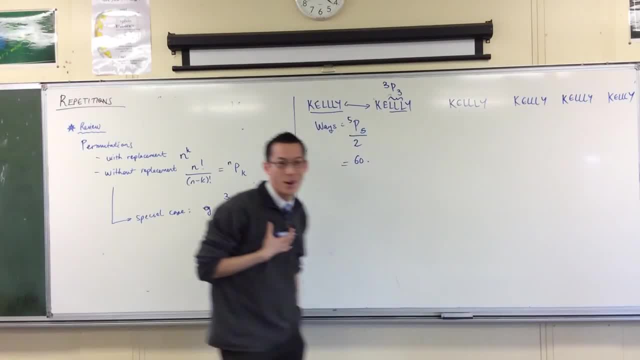 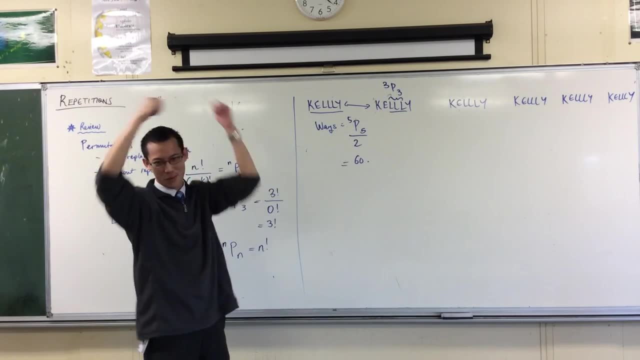 There we go. Okay, Suppose we were, you know, really good friends in the family. We actually knew how to tell them apart. You're like, oh no, That's the one with the scar And that's the one with the left part, not the right part, or something like that. right, 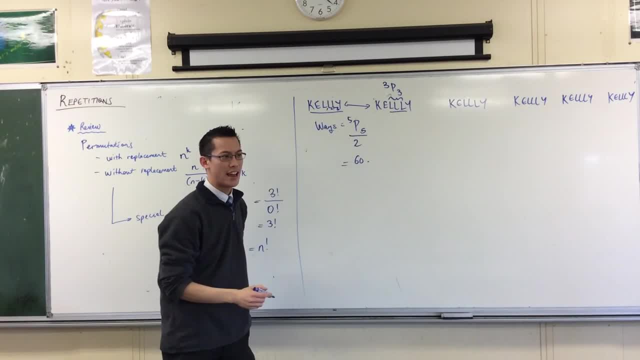 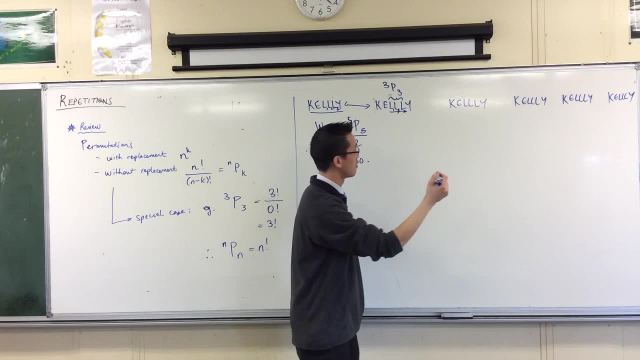 So you're like, I know which ones- first, second and third, right? So now that you know which ones they are, you can tell them apart. You know this one might be, say, one, three and two, right. 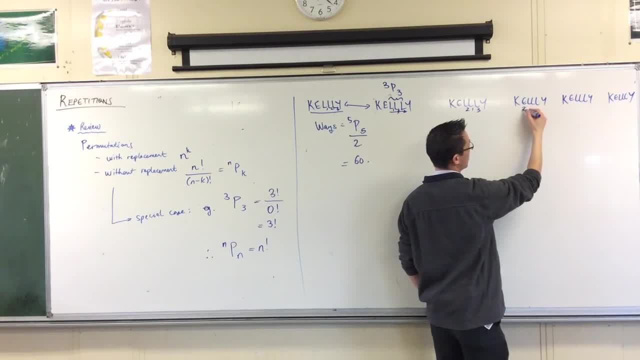 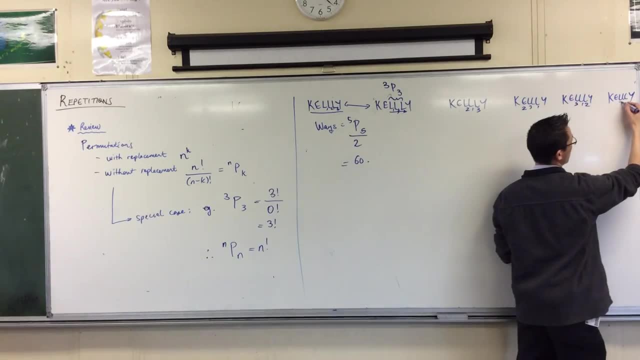 Maybe we can put two first, Two, one and three, Two, three and one. I'm off, You get the idea. And then three should come first: Three, one, two, Three, two, one. Okay. 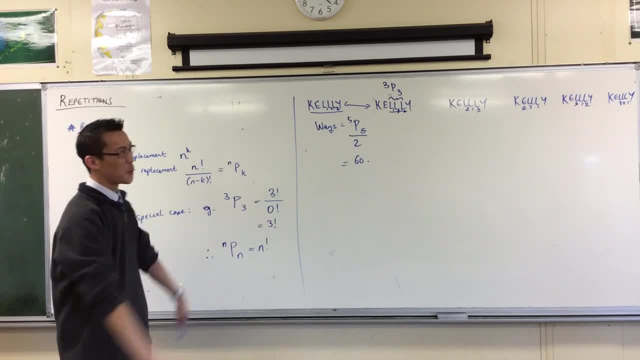 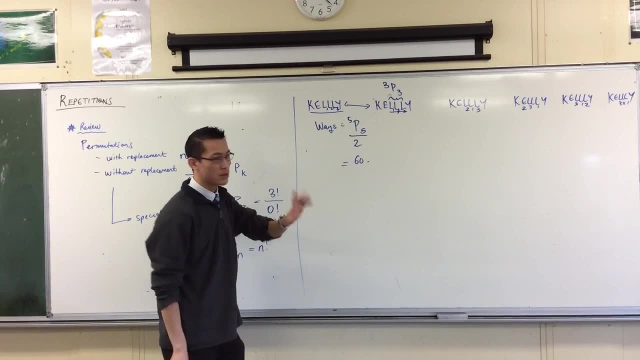 So the triplets can tell, but we can't. It's all the same word to us. Okay, So I've overcounted by this factor. Does that make sense? All right, So therefore, you know, this is example one. 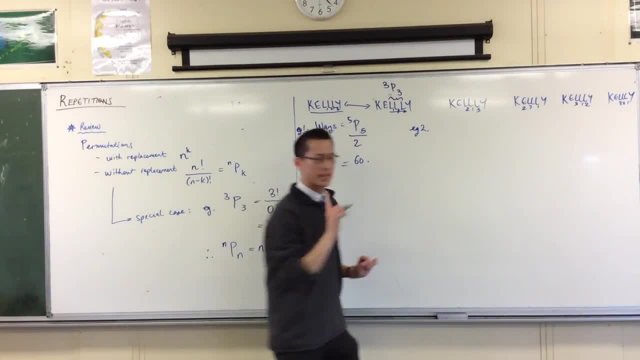 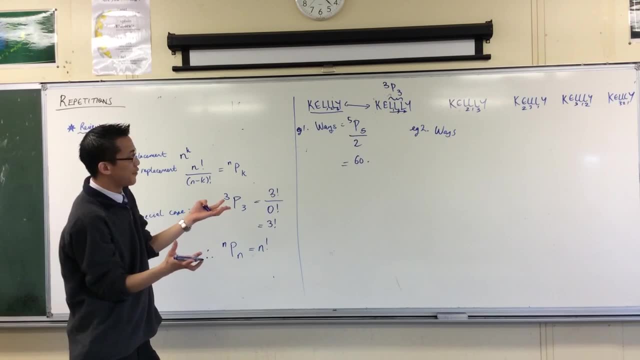 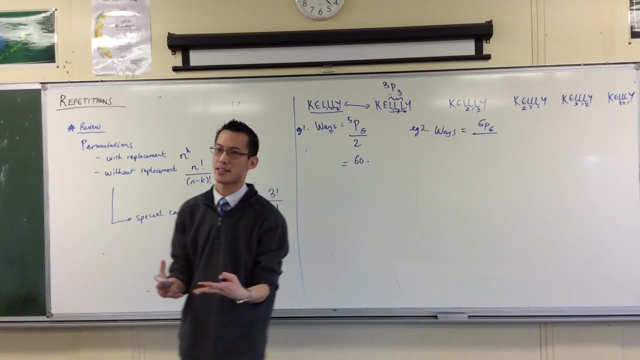 Example two. it starts with: what's the numerator? How many letters do I have to choose from? I have now six to choose from, because I added an L right, So I've got 6p6 on the top, But then I've overcounted by this three factorial right. 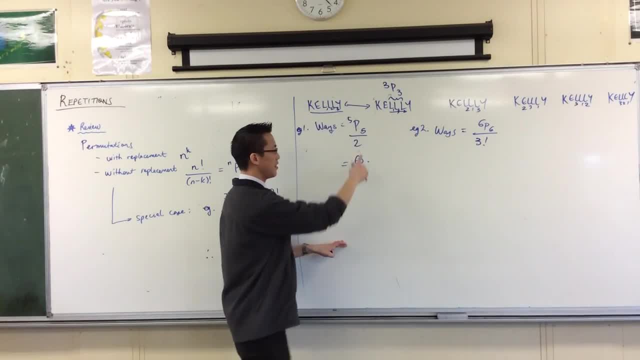 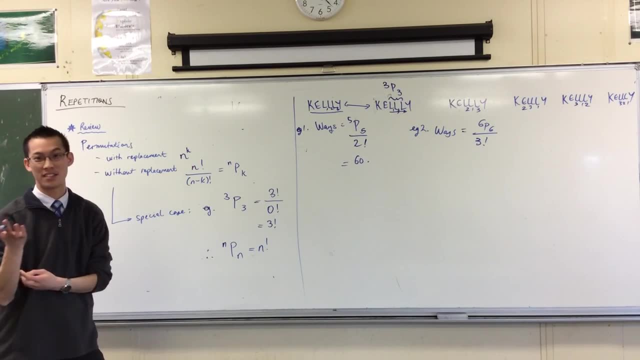 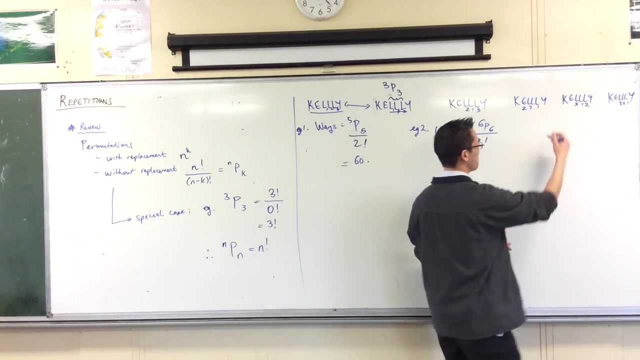 So really it's easier to see with three, This should actually be two factorial. Does that make sense? Because it just happens to be a coincidence that two factorial is two, right, I guess, if you wanted to think about it this way, let's go one more. 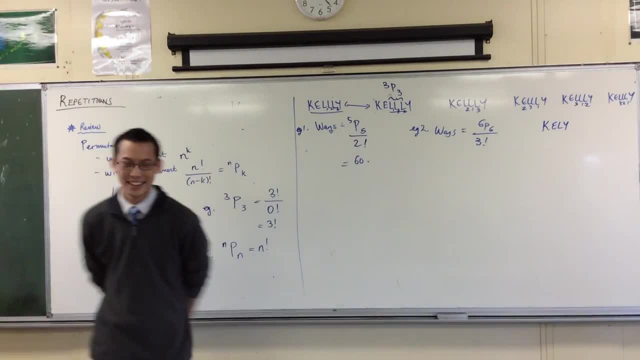 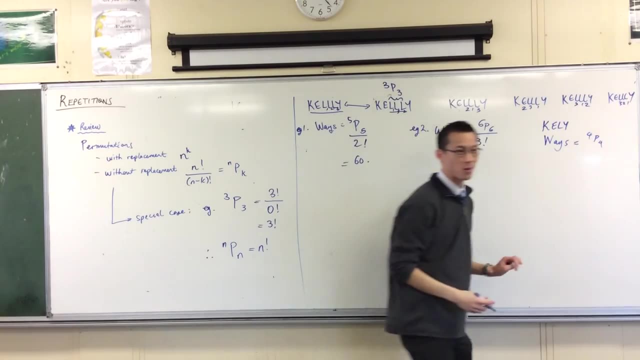 Suppose, instead of adding an L, I chopped off an L. okay, Now let's think about this: How many ways are there? Well, it's 4p4 on the top right Now, if you wanted to push it, because we're generalizing here. 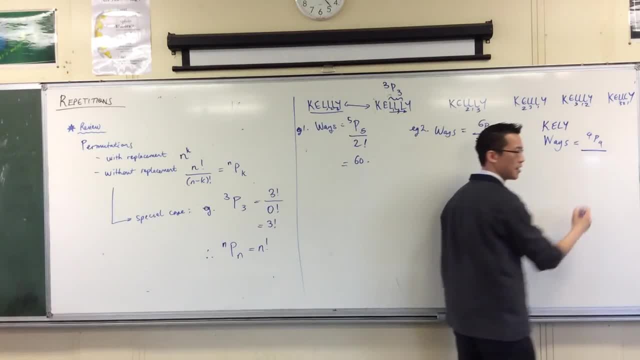 We're trying to see this right. You've got four letters right, Four letters, And so you've overcounted by a factor of one factorial for the first one, and then one factorial for the second one and one factorial. 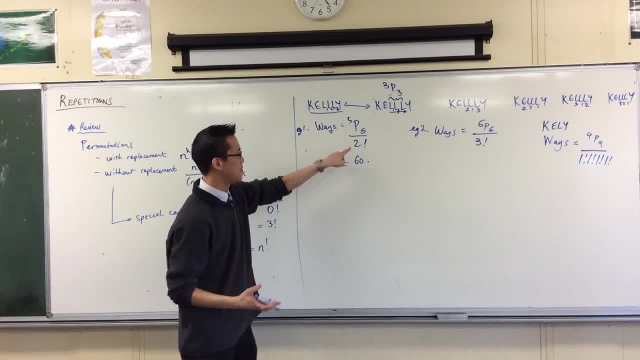 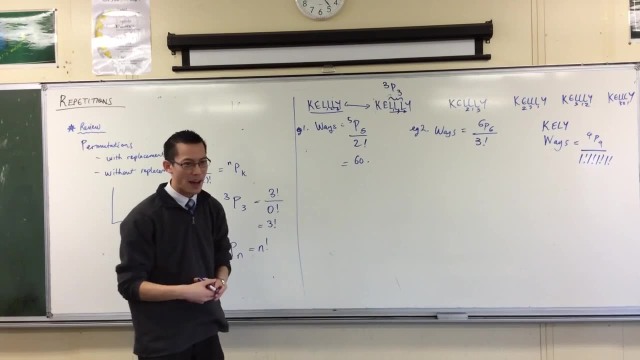 So I've got four different letters, right. It just so happens that in these cases, this is how many I've got of those different letters and the one factorials don't matter. Okay, But sorry, I'm just going to keep on doing violence to your name, if that's okay. 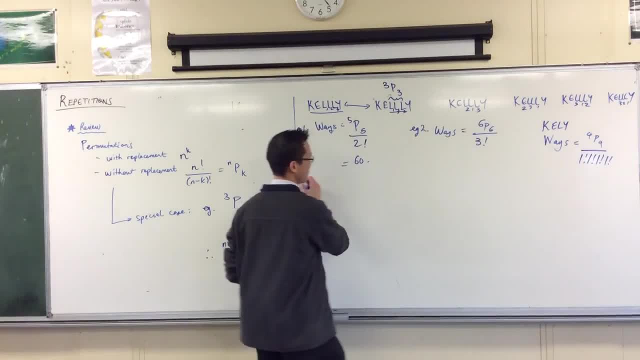 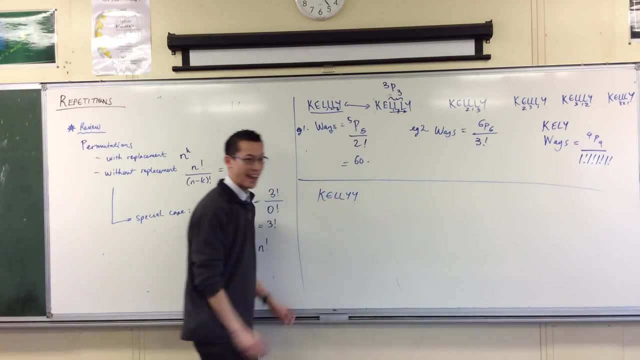 Let's suppose I'll leave that one there. You know too many L's. that's a bit mainstream, okay, So instead I'll leave the L's and I'll add a Y. okay, Right, So so ways. okay. 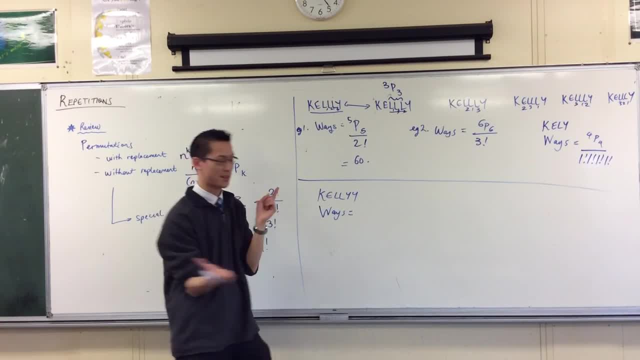 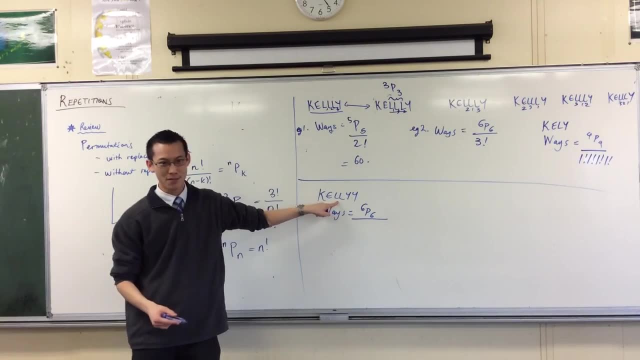 How many? in total Six. So there are six p6, six factorial ways. okay, Now, Now you already know that L's can switch, right, So you've overcounted by a factor of two. factorial, okay, But the Y's can switch as well, totally unbeknownst to the L's, okay. 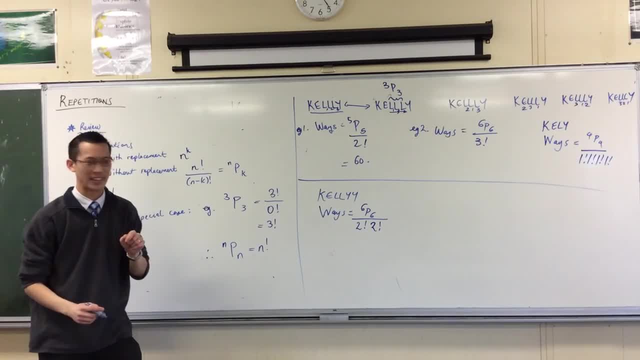 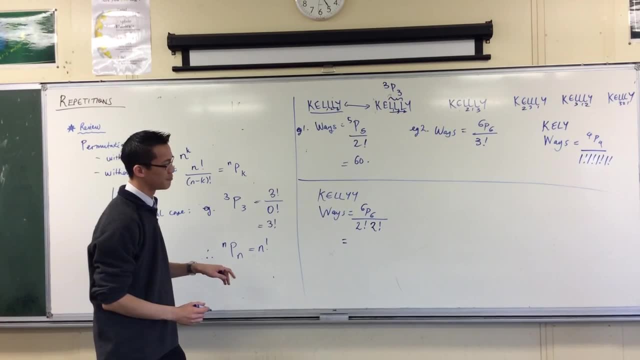 So you've overcounted by another factor of two factorial, okay. So I don't know- six factorial on four. I don't know what that is, but you can work it out: 720 divided by four, 720 divided by four. 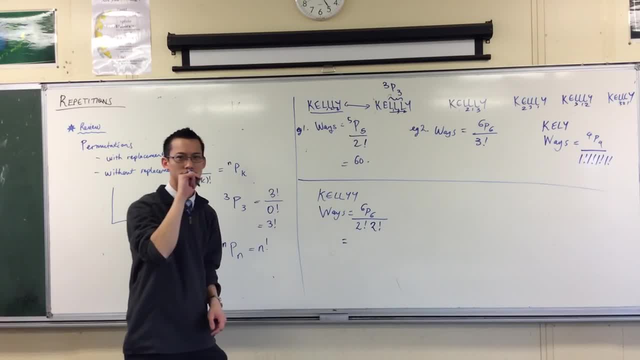 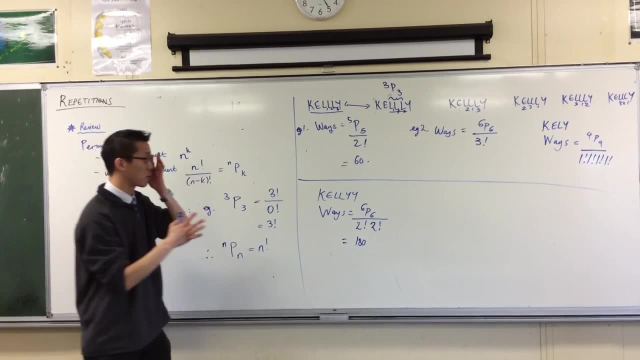 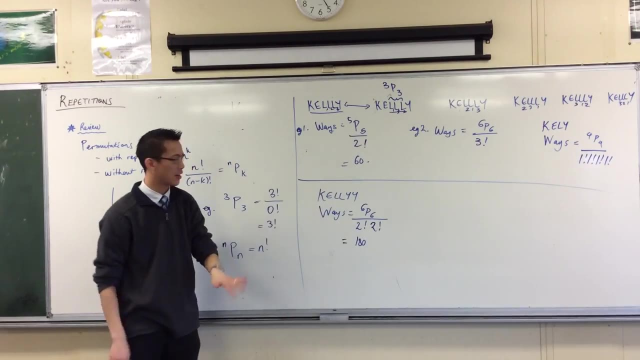 What's that? Eight, 180.. 180?, 180.. Okay, But you get the idea. It's this very simple concept that you know. however many repeated letters you've got, and if there's one, that's the scenario, that's what you'll have, okay. 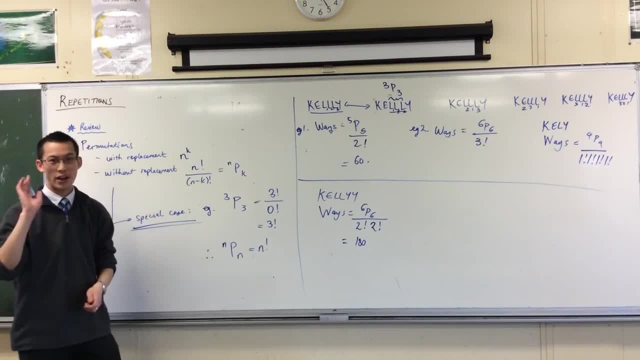 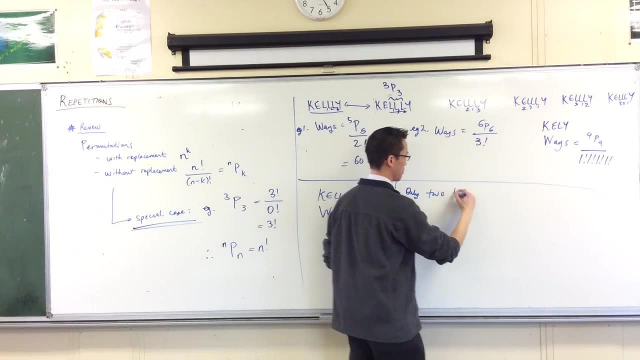 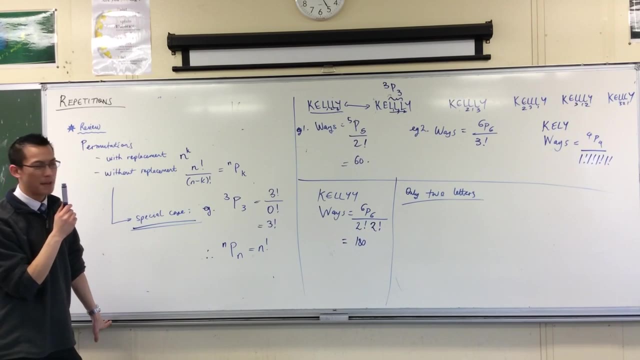 Now we started this off by looking at a special case. We're going to look at one last special case and then I'm going to stop talking. Only two letters, Okay, Okay, Right, So now we're being totally, totally hipster, okay. 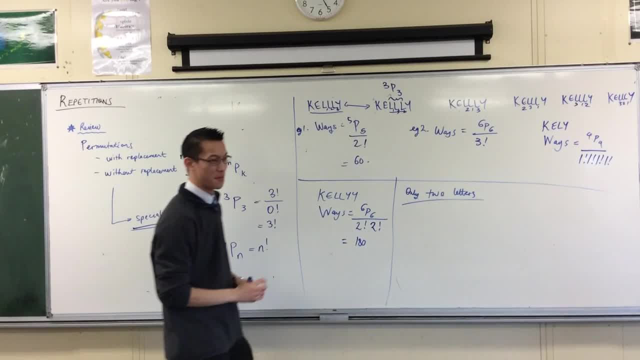 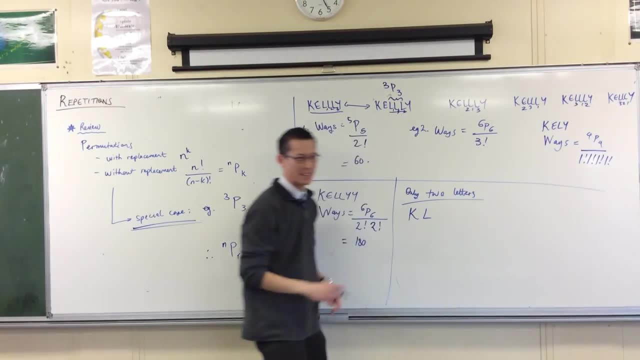 You know, there's all these alternate spellings for names. okay. So I'm like really, really weird, So I'm just going to leave out all of the vowels. okay, So I've got a K and an L, but I'm like two letters that's not enough. 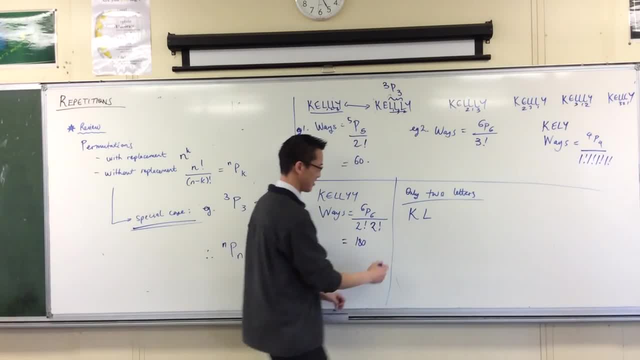 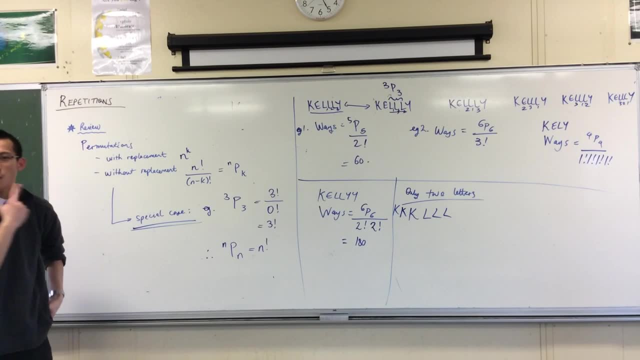 You need something more substantial for a name. So I'm going to add on more K's and more L's, and one more for good measure. Okay, there you go Now. how many ways to rearrange this. How many ways. 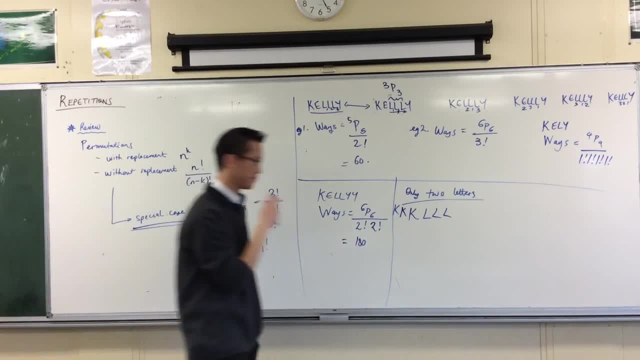 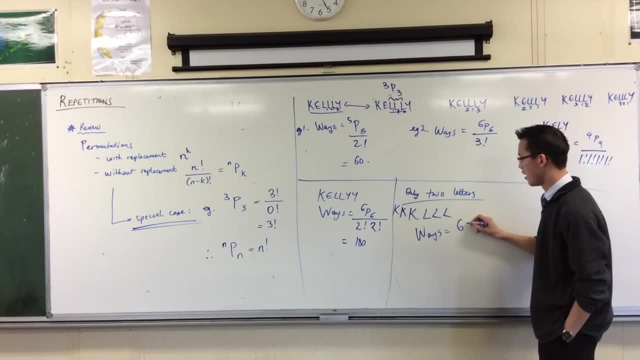 How many words? Okay, Well, how does it go? So the number of ways you already know? by now you're going to have 6P6 on the top. Okay, I'm going to stop writing that in permutation language. 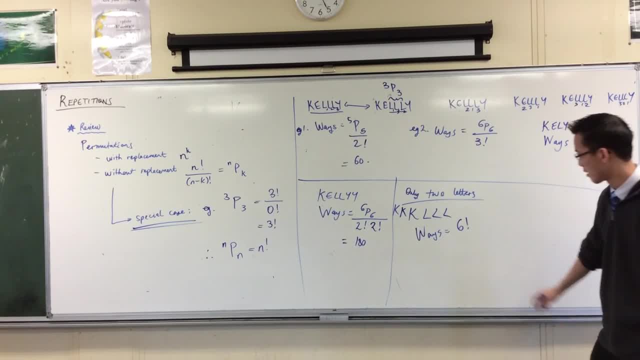 I'm going to say it's 6 factorial, because we've already established this. Now, how many repeats are there? There's this set of triplets that can all switch and we don't know the difference. And then there's this set right? 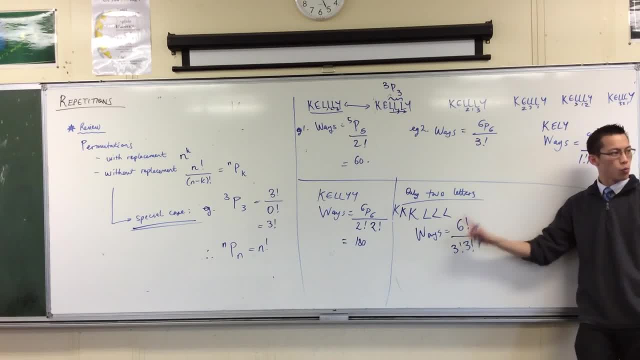 Now, this one is interesting because I mean, you can work out what the number is, but this is a pattern that I'm familiar with. okay, It's not just 6P6 divided by some random thing. I can write it in a way that makes it a little more obvious, okay. 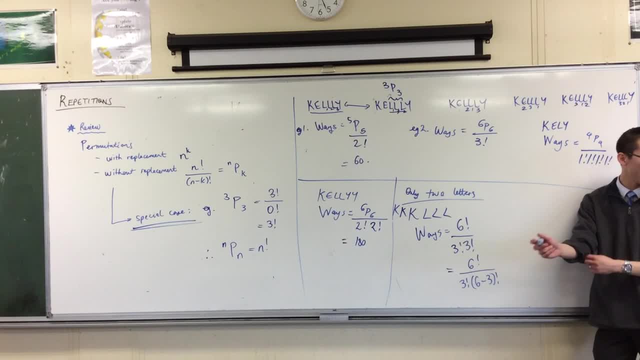 Where have we seen this? We've seen this recently. right? This is binomial, isn't it? This is this. This is not 6P, This is 6C3,. okay, Now hold on a second Stop. 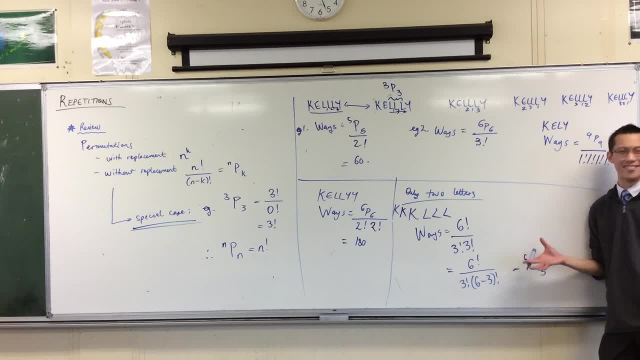 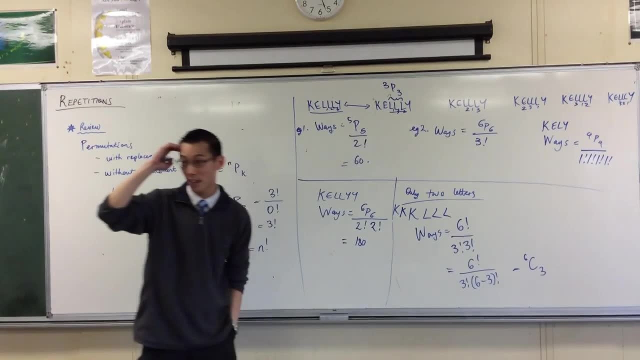 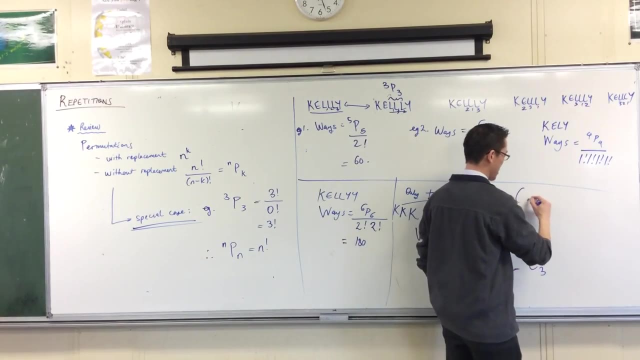 Why? Why, after mangling Kelly's name this far right, Why have we ended on binomial theorem? And the answer is: well, how many letters do we have again? We've got two letters. You know, something like say this: 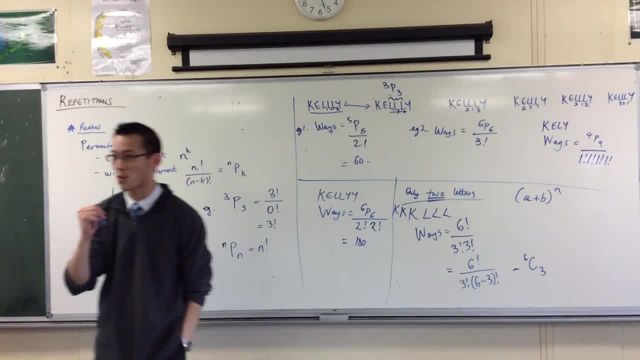 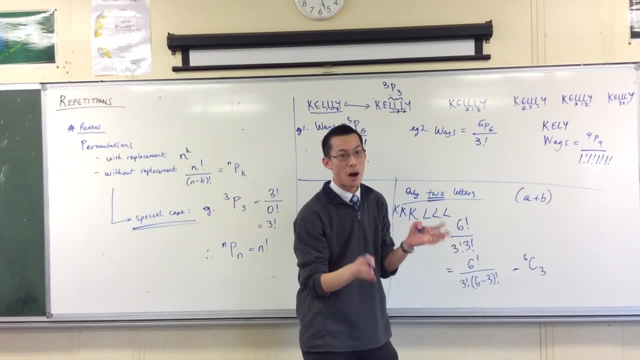 You've got two letters to choose from right, And every single time, Let's just think about an expansion of this right. Think about an expansion of this. Let's pick out- I'll pick out- a number that's manageable, right. 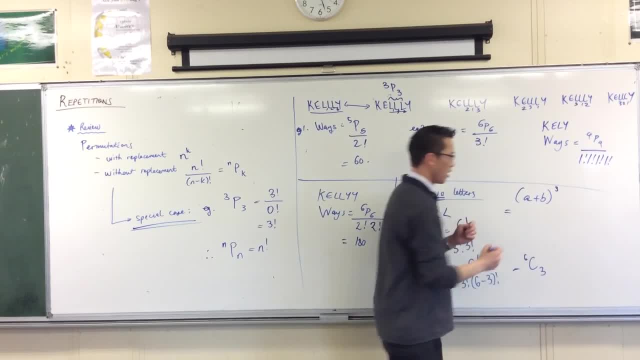 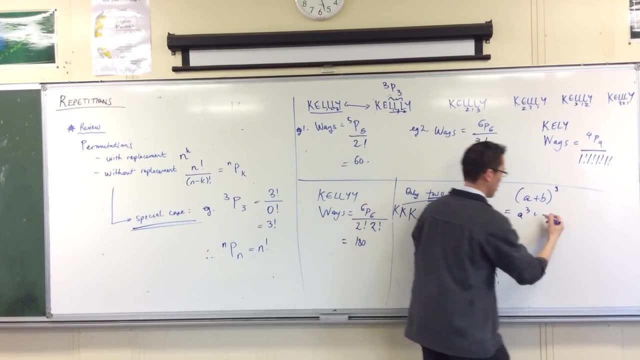 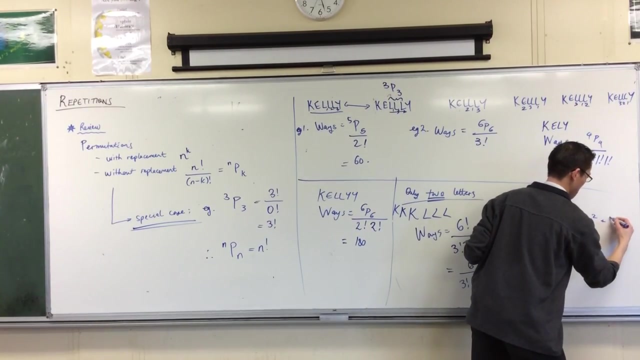 Like say, let's go 3, okay, What's the expansion? We know this. back to front, right, What's the expansion? We've got A cubed plus 3A squared B plus 3AB squared plus B cubed. 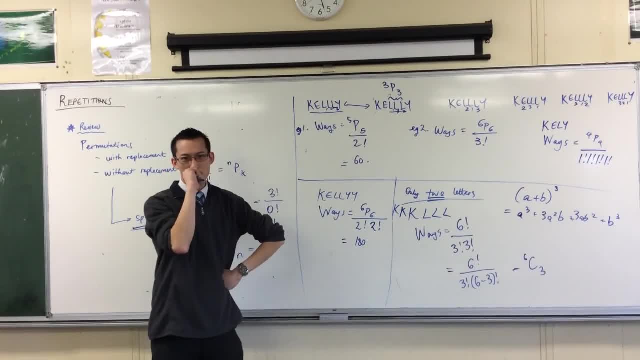 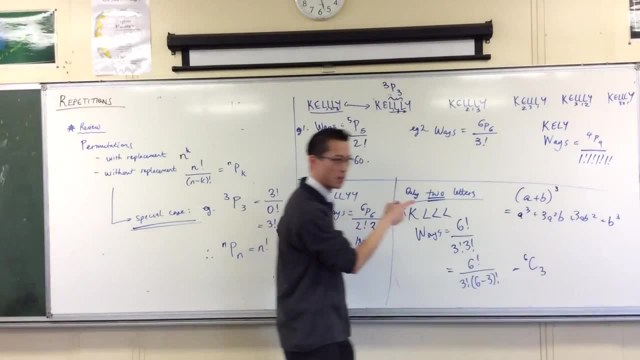 Yes, Okay, Now hold on a second. This looks like it doesn't have all that much to do with what we're doing, but it does. right. These are words. Look at them, They're words. Here's one. 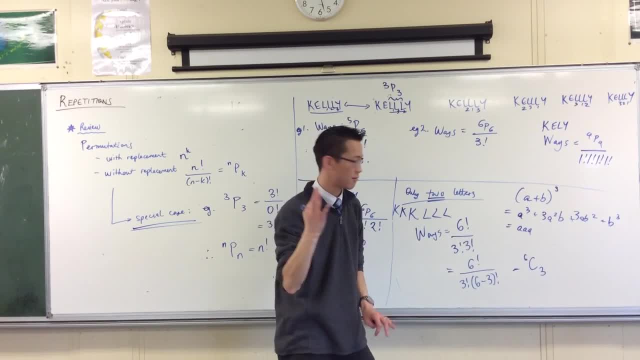 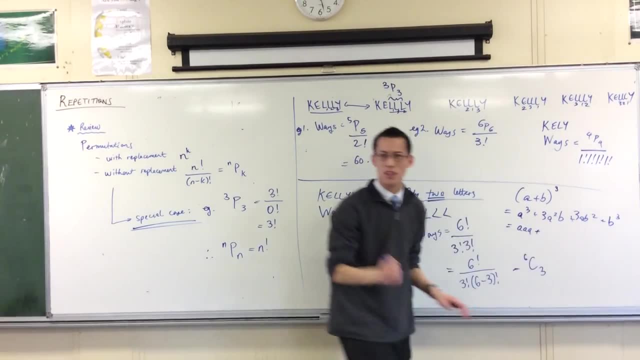 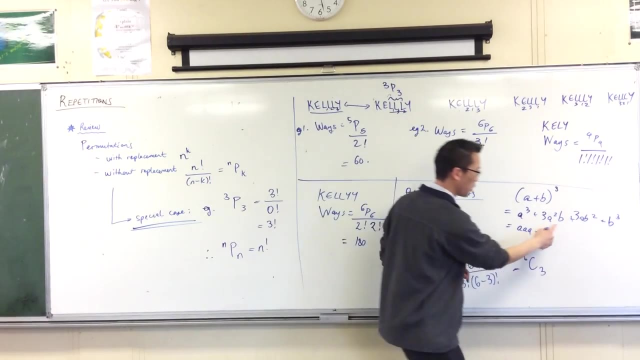 A, A, A, It's a word. Three letters right, And I had two to choose from right. Now, what about these guys? Hmm, Why are there three there? Why would there be three? And the answer is because I can arrange two A's and a B in three different ways. 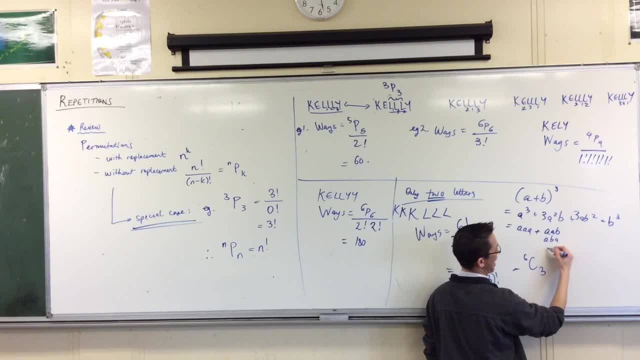 Namely: I can do A A B, I can do A B A And I can do B A A. Look, there's three of them, Three arrangements. You're going to repeat it over here, right? 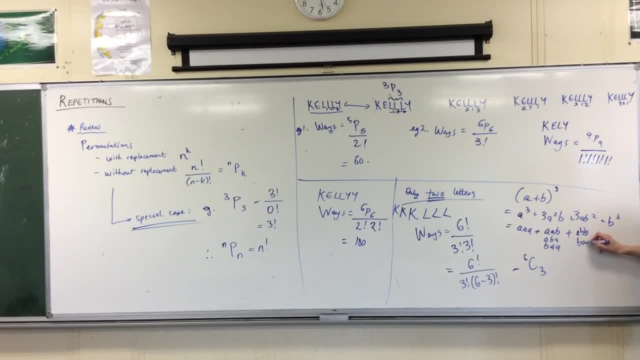 You've got AB, You've got BAB And you've got BBA- Okay. And then you've got your last one OVA Here, Okay. So hold on a second. The thing is right. you know what all of these numbers are right? 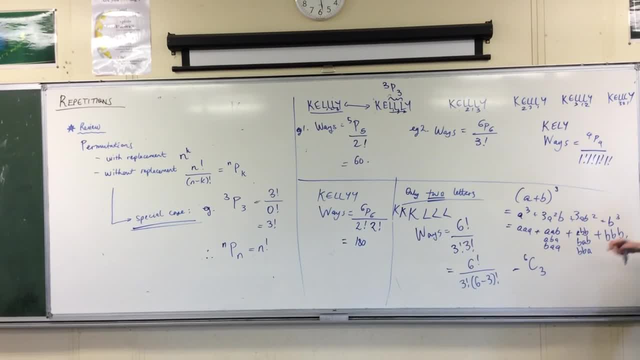 These binomial coefficients. binomial coefficients, they come from arranging pairs of letters, right? What's this guy This is? I'm running out of space and I need a new car. This will do, Okay. One One, Right. 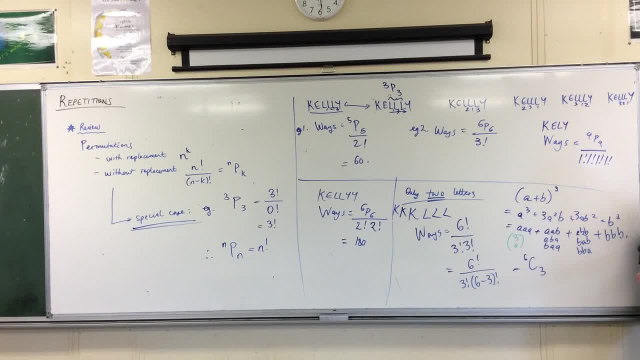 It's three choose zero, isn't it? Three choose zero? Why is it three choose zero? Because how many ways are there to arrange three letters that are all identical? The answer is, well, there's one way, right. And then here you're going to go: three, one right. 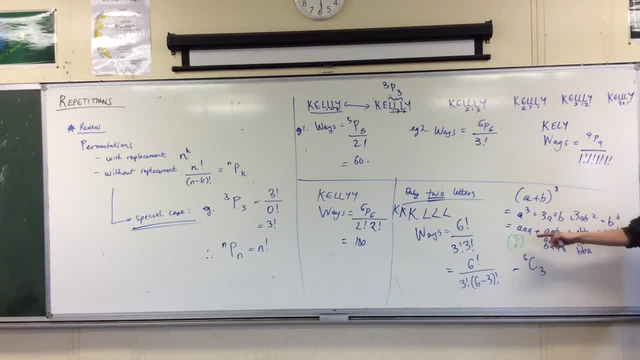 And then three, two, And then three, three. Now, what are the zero and the one and the two and the three? It looks to me like it's the Bs, right? How many Bs do I have to choose from here? that will mix things up. 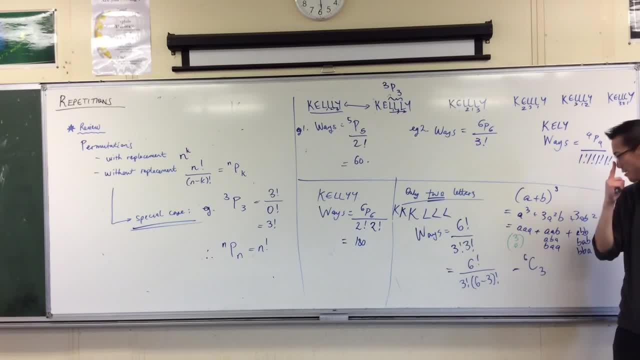 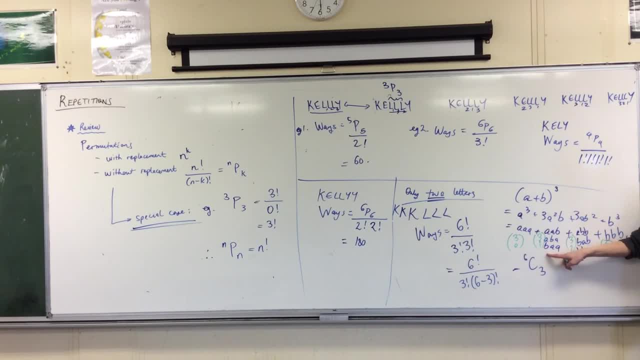 The answer is: I don't have any Bs. Here you get one B, and that mixes things up. here you get two of them and here you get three of them, which puts you back in the same position you were at the start. Does it make sense? 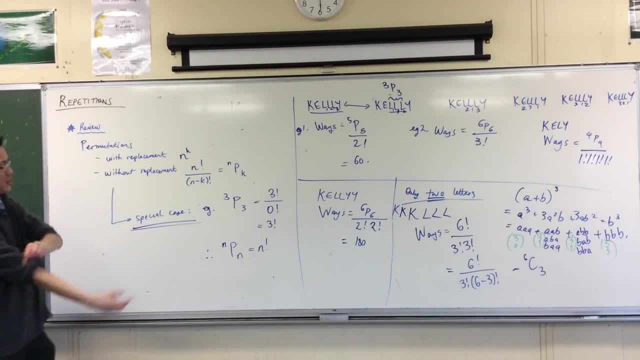 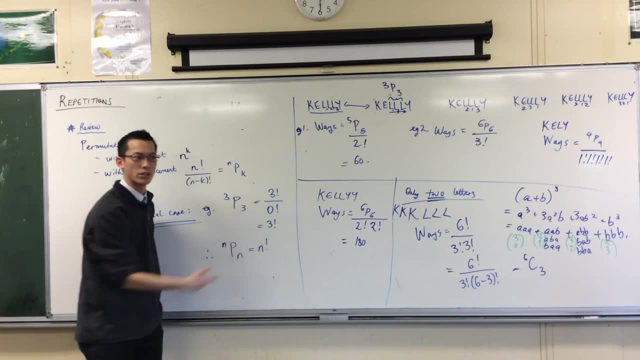 Right. so the big ideas were: 1. If you are arranging without replacement and you want to arrange No Big idea, okay, No. 3. all of the objects you've got, you just get n factorial. That's the first idea. 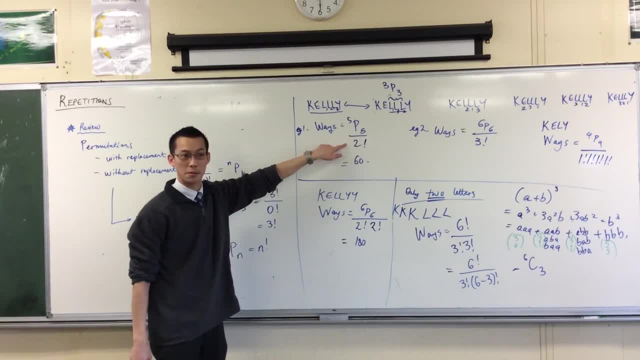 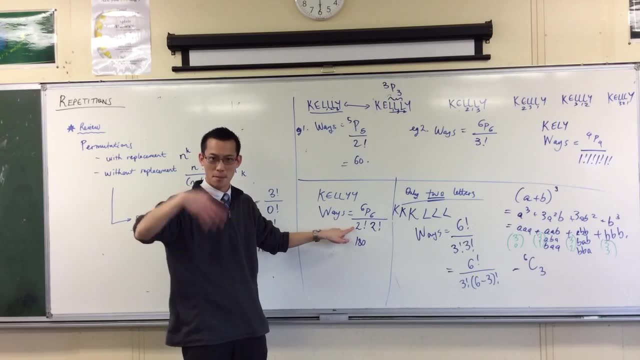 The second idea is when you're repeating them, you're over-counting. So however many times you over-count, you divide by that factor to fix up the actual number of arrangements. get rid of all the repeats, get rid of all the times. where you can't tell the triplets apart.